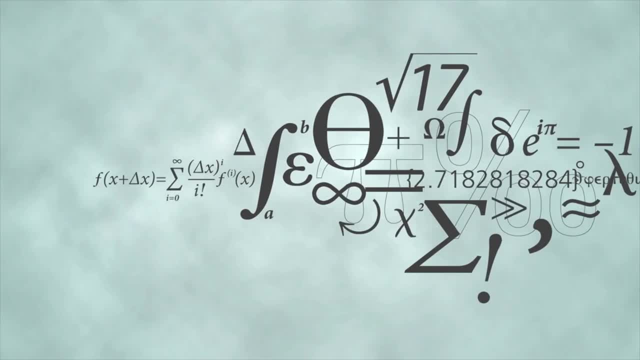 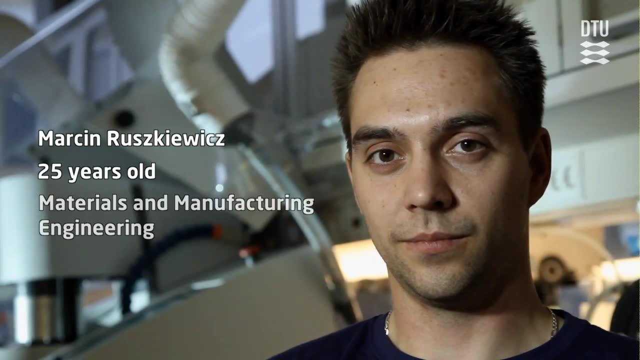 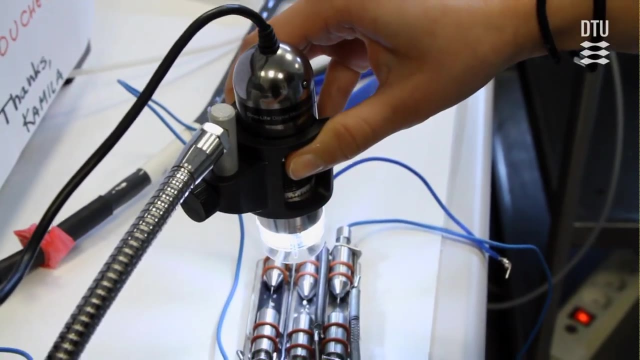 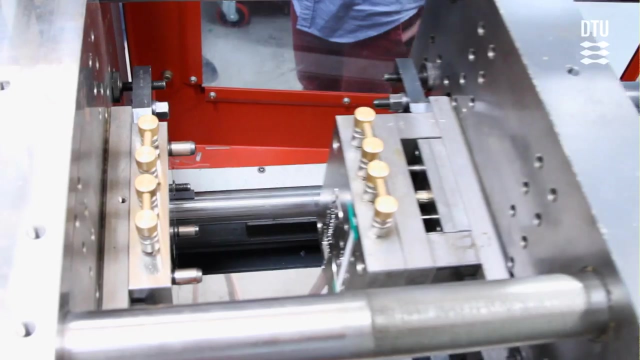 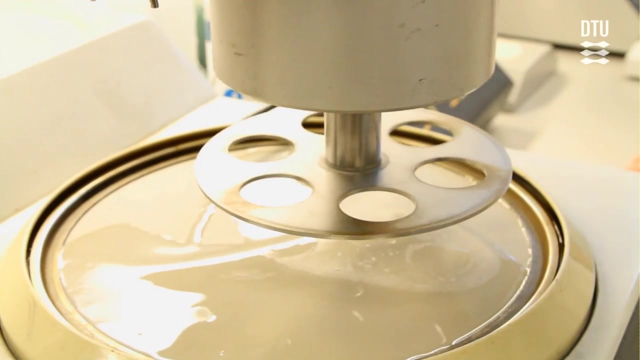 My name is Marcin Ruszkiewicz, I'm 25, and I study materials and manufacturing engineering. My first contact with DTU was during my last exchange. Then I decided to come back here for my master's studies, So I did my bachelor at the University of Technology. Then I arrived. 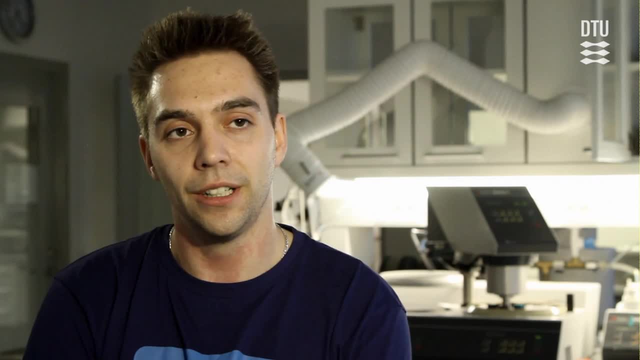 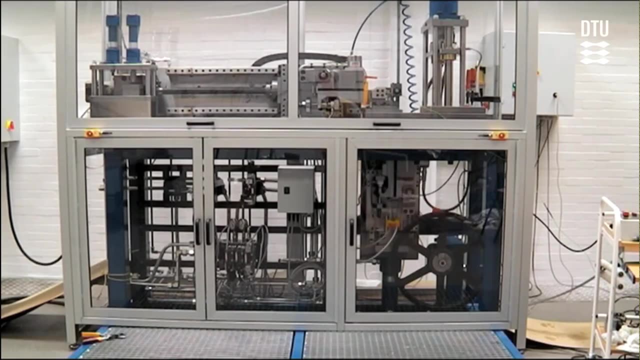 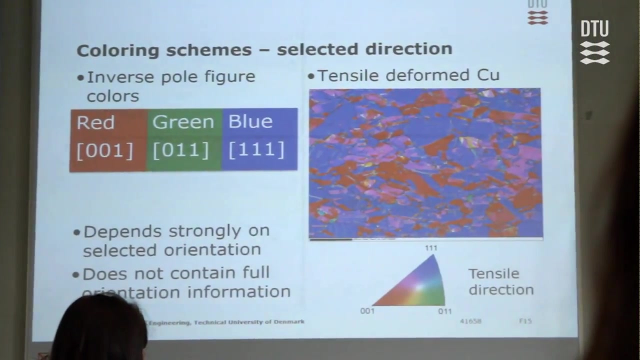 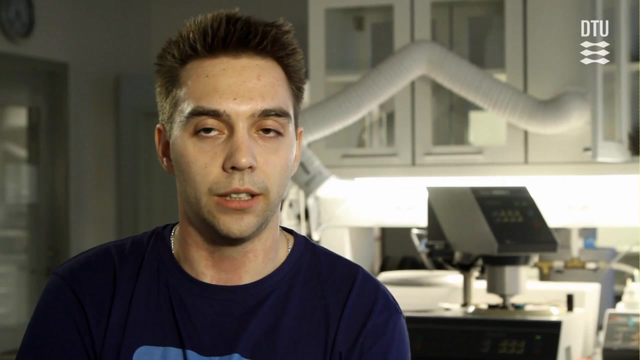 here again. here I was studying for one year, Then I moved to the US for my master's studies for one semester and now I'm back here. Frankly, DTU is the place where I've never had more contact with the equipment myself. 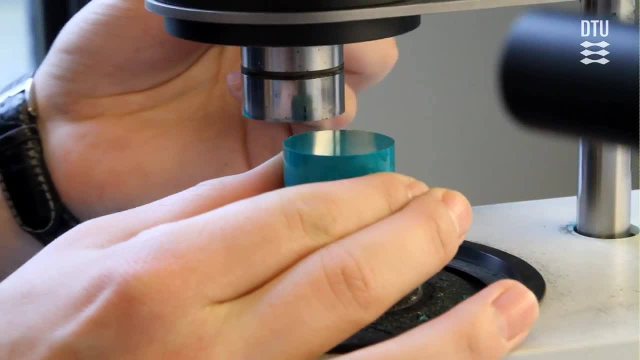 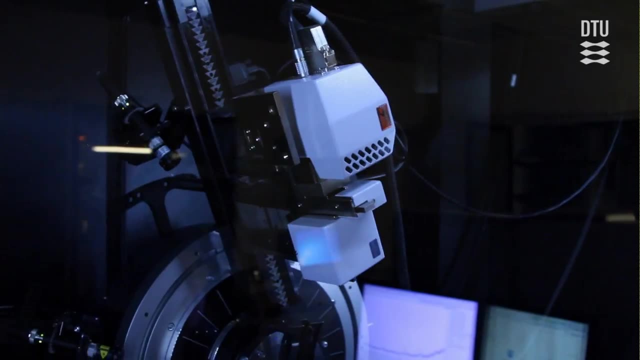 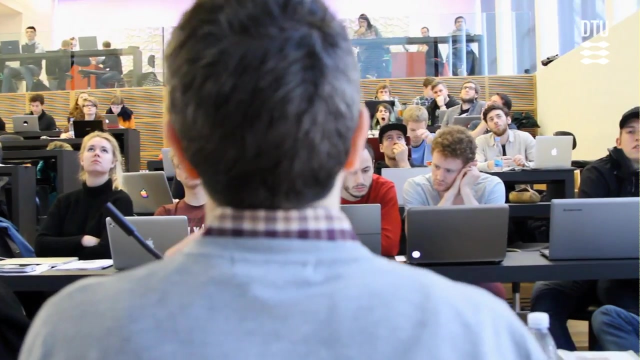 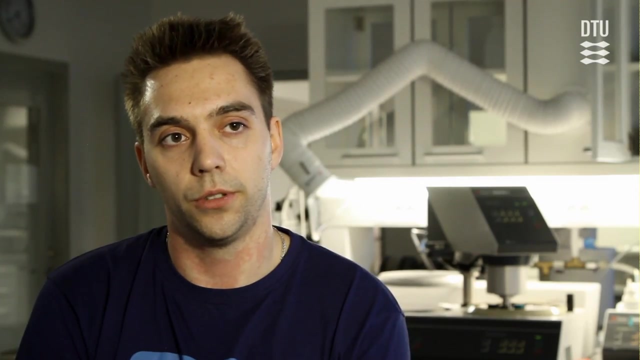 I prepare my samples myself, I polish them. I had the opportunity to work with microscopes, have hardness tests, a lot of things. It's really, really important You have very good cooperation with professors. It's a really personally oriented approach. 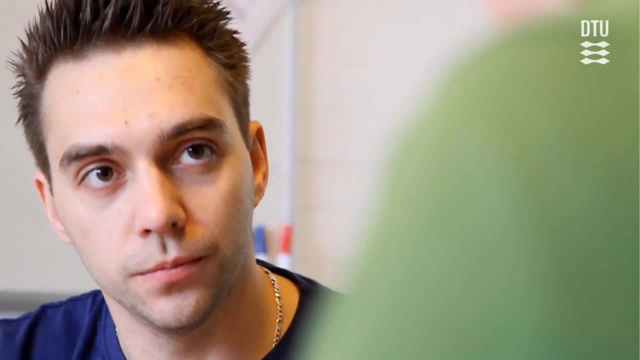 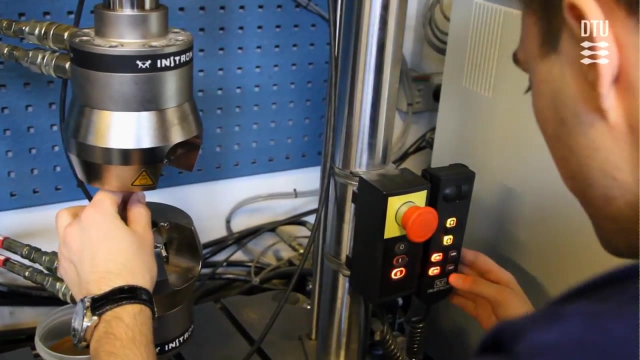 In my master's I work on copper. We investigate the polycrystalline of the copper, how the microstructure, exactly the substructure, develops when we cyclically load it. It's a lot of fun when you can do something yourself. 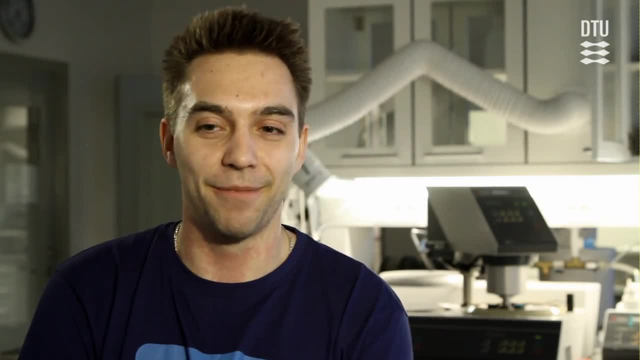 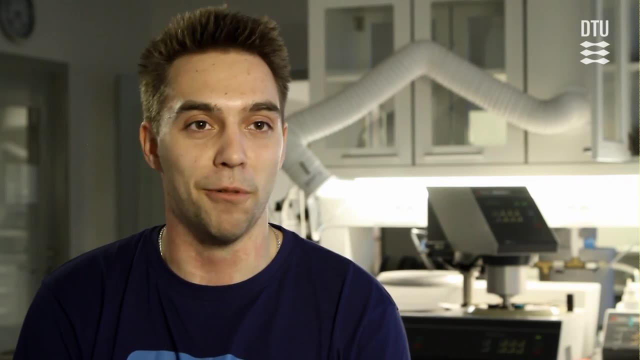 You work on something the whole day and it doesn't work. For example, I was working on my samples to prepare the experiment and nothing was going as I wanted it to. But once it works And you start getting results you wanted to. 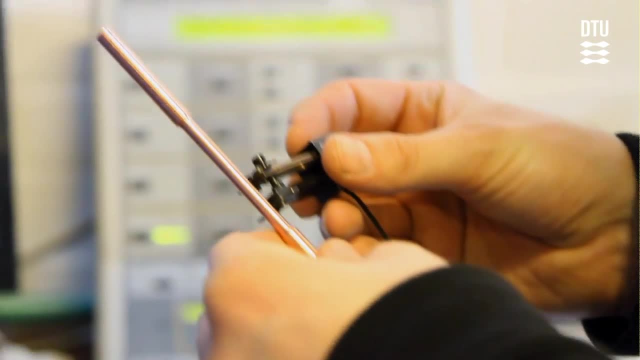 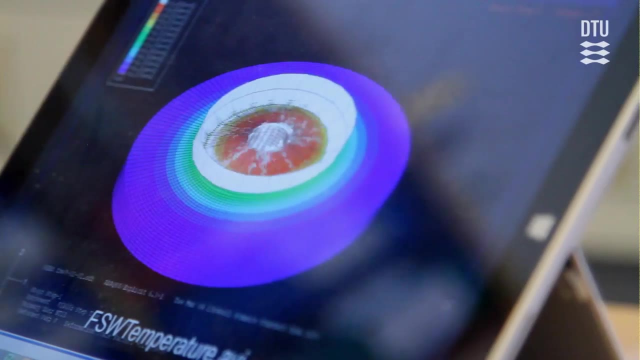 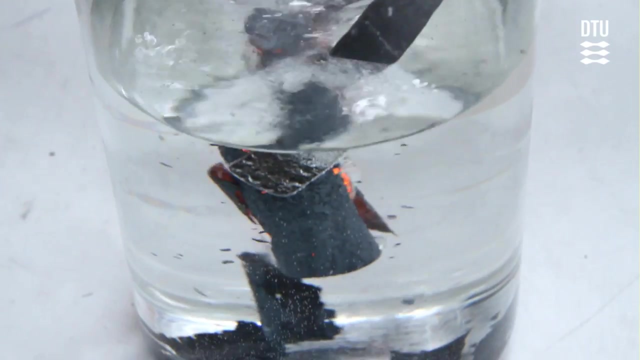 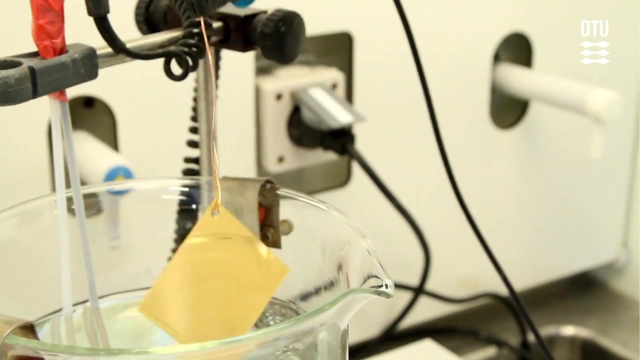 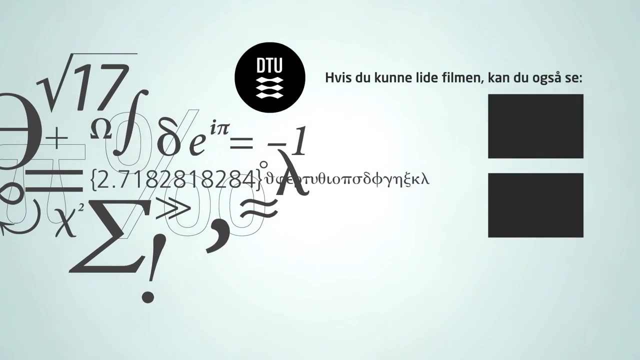 Then you feel like I'm improving, I'm investigating something. I believe this is the most fun part of it And obviously all the student life we have here. It's a lot of fun.